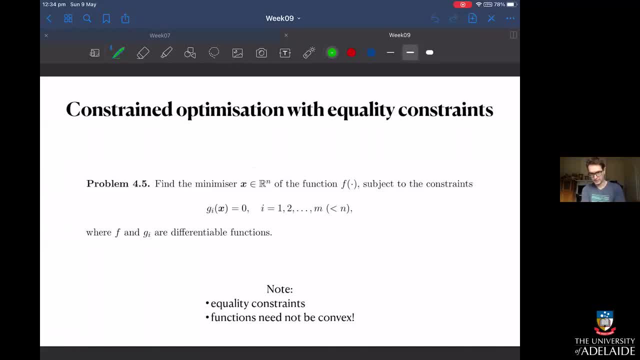 examples of problems with Lagrange multiplier method, with equality constraints, and I'll talk through a couple of them, and I'll leave most of them for you to work through yourself, because they're well described in the notes, and then we'll have a little bit of a talk about what the 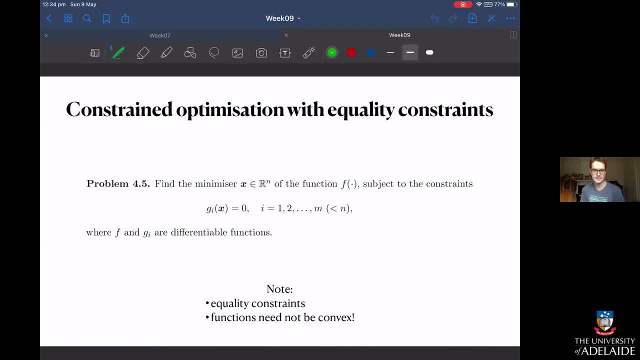 method is. So here's the problem that we're trying to solve. So this is a constrained optimization problem with equality constraints. So you're trying to find the minimizer of some function, f, that's subject to the constraints g. i of x is equal to zero, So that equals sign is important there, right? so that's. 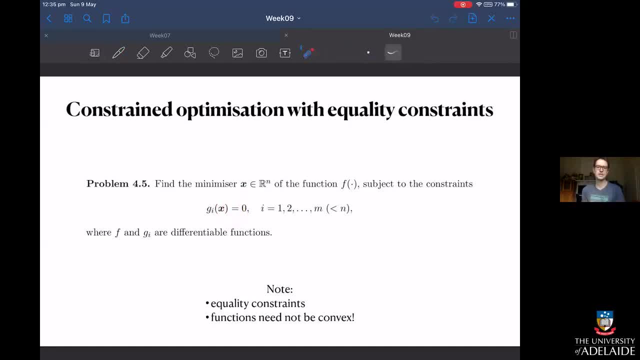 the equality constraints and you have to exactly match those constraints. So f and g are differentiable functions here. Note that those these functions don't actually need to be convex right. like and unlike what we've been talking about in previous videos, we don't actually need the functions to be convex here, they're just 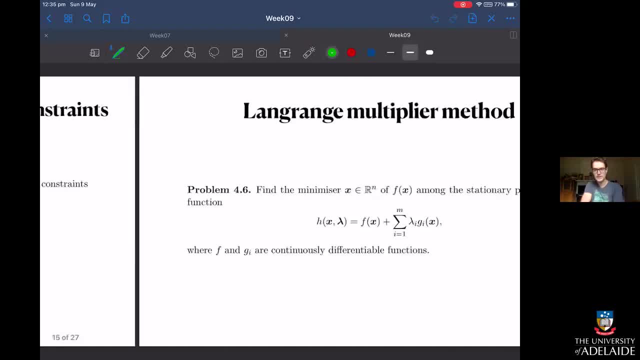 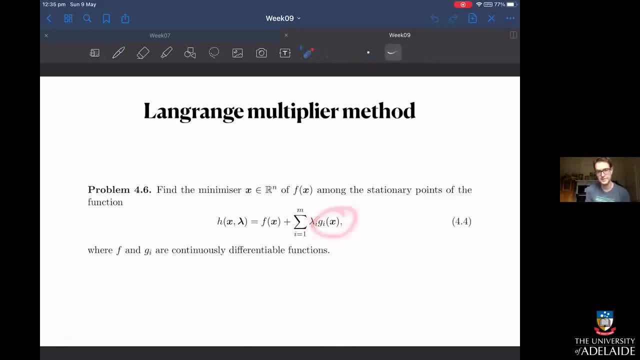 it takes these, these gi's that all have to be equal to zero, and then it creates a new cost function h, where basically I tack these equality constraints onto the end with some new parameter in there that's called the Lagrange multiplier right, and so the idea of this is that if I'm trying to 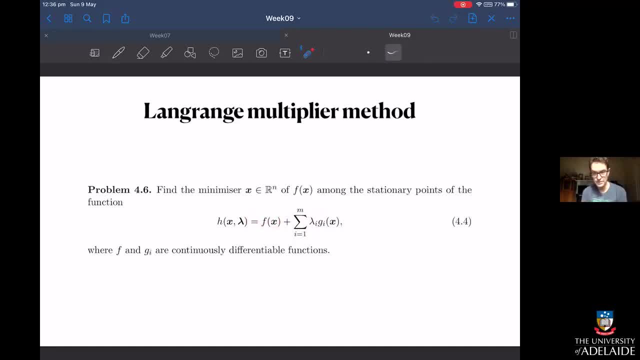 minimize these f of x, f of x. if I want to demand that these equality constraints are satisfied, so the so that each of these GIs of X is equal to zero, then I should be able to tack them on and the minimizer of this function should be the same. 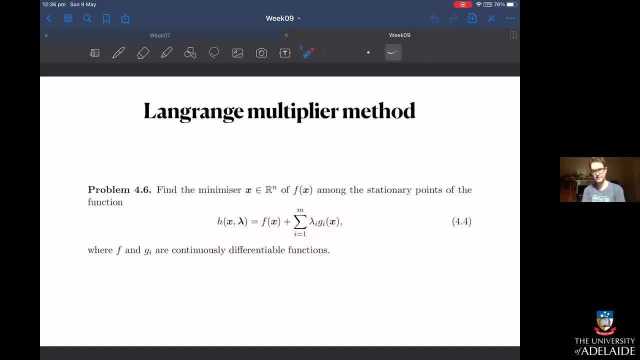 as the minimizer of the F function with these constraints here. So really it's exactly the same problem. I've just added on my constraints into this cost function as an extra term. Okay, so here's an example of this, And so this is actually the sort of problem. 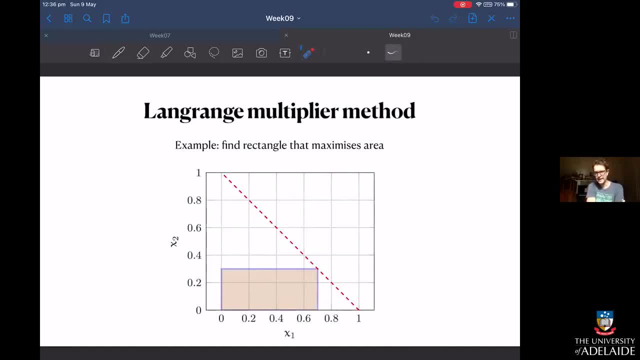 that you've seen ever since you've been doing differential calculus, and the Lagrange multiply method is just a new formalism for solving these things. So here's a classic example: find a rectangle. I find the rectangle that has the maximum area, given that the rectangle has got to sit underneath. 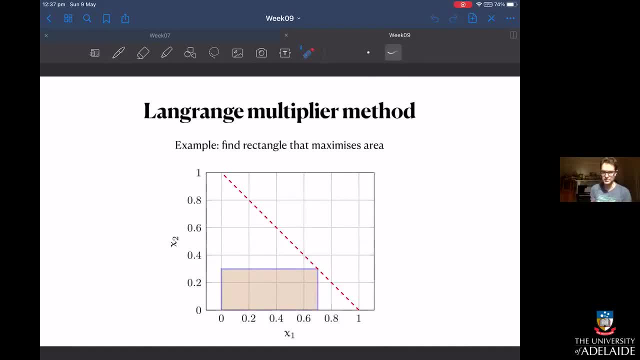 and the square here. So this is the sort of problem that you've done, building a fence and sort of things that you're going to be able to solve with this problem. So you've got a little bit of a different constraint here, The constraints on the amount of perimeter that I have. 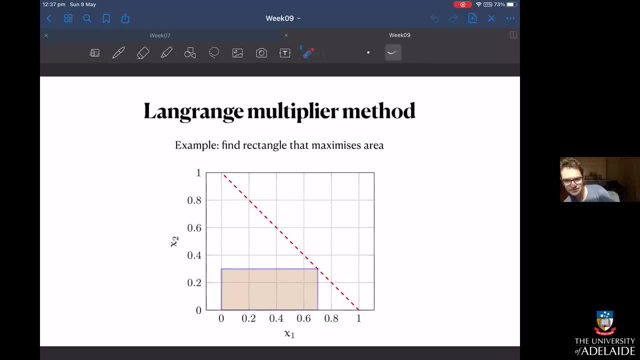 I have to have that. these points sit on the edge of this line here. So you might expect, even without doing this problem, that it's likely in these sorts of problems that you're going to get the optimal solution. It's going to be something that looks square, like right. 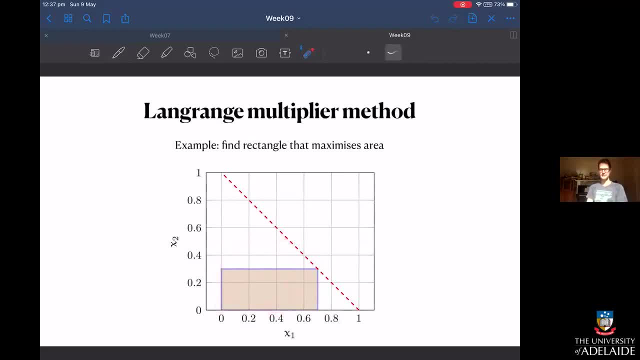 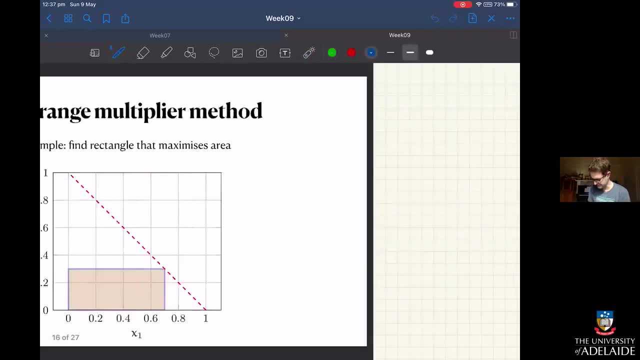 Like the square of this area is. you know, we tend to like, like those sorts of solutions And that's what we'll, that's what we'll find here. Okay, so how do we do this? So what are we trying to do here? 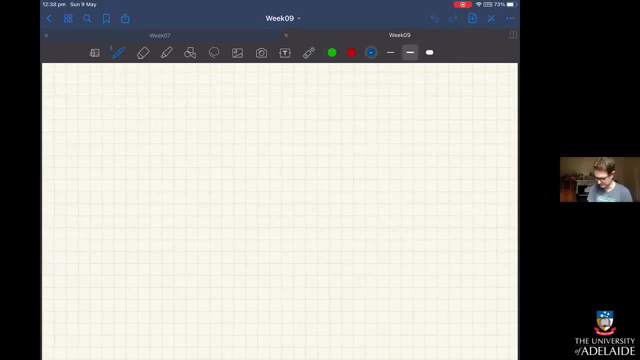 So the, the size of the rectangle are going to be these distances, these lengths: X1 and X2.. And so the problem is, we're trying to find the maximum area. So instead of maximizing the area- because in this course we like to minimize functions- 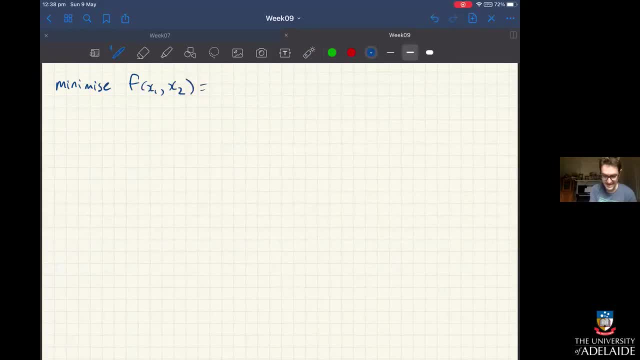 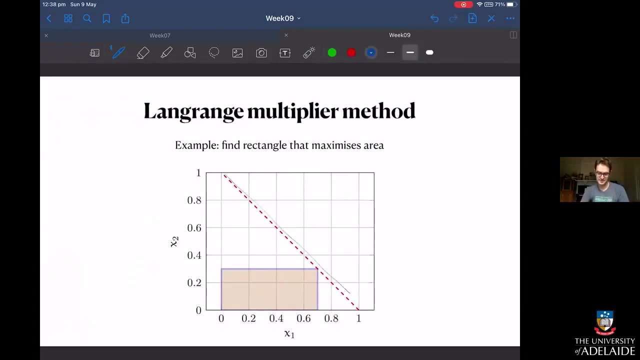 we'll minimize the function X1, X2, that it's the negative of the area, right? So minimize that subject to subject to, and the width and the height of these have to lie on this. You have to sit on this line here, right? 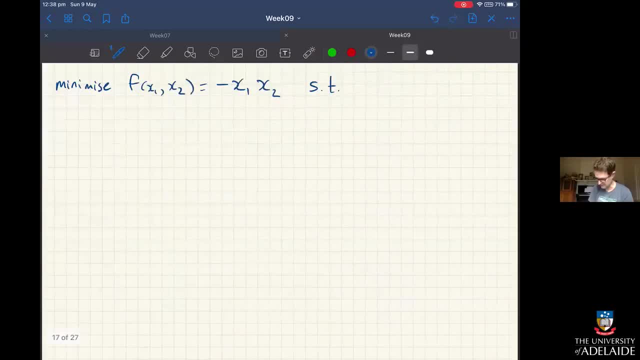 On this, on this line, And you can figure out the equation of that line, which is going to be that X1 plus X2 is equal to one, And I don't want to have negative solutions here. So X1 and X2, both. 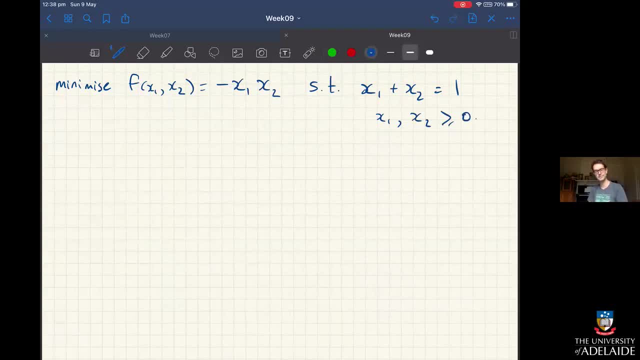 got to be greater than or equal to zero. So that's my problem, right? So I'm minimizing this cost function, that's, the area subject to this constraint, such that the width and the height of this thing have to lie on that line: x one plus x two. 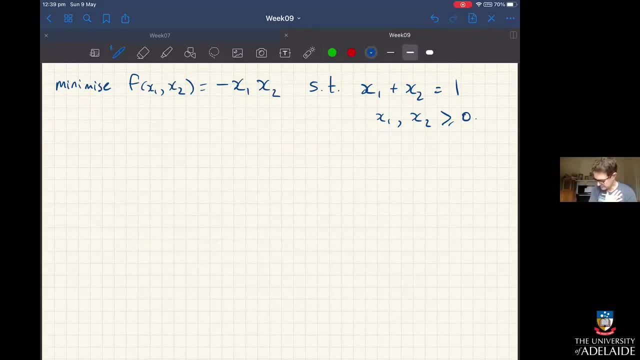 x plus y equals one right. So how do we do this with the Lagrange multiplier method? So what we do is we take our function f of x and we create a new cost function that's got a lambda in it. now that lambda is gonna represent our constraint. 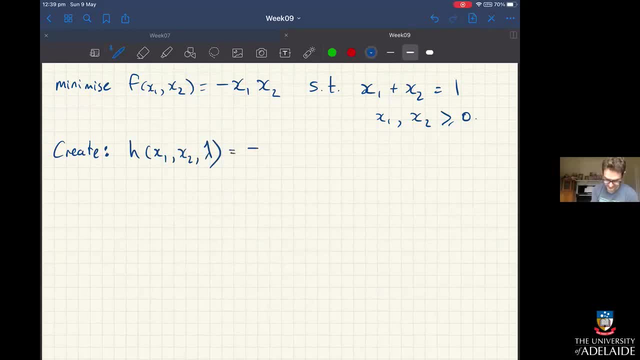 So this is going to be f of x one x two. f of x one x two is negative: x one x two plus lambda times, my constraint right. So this is gonna be lambda times: x one plus x two. take away one and multiply by lambda. 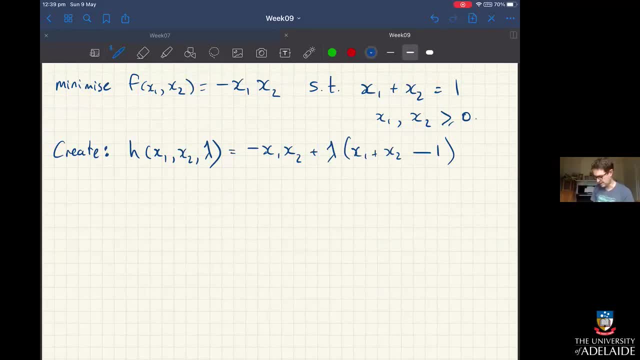 That's so. that's my Lagrange multiplier function. And now the method says the minimizer of this is going to be when dh dx one is equal to dh dx two is equal to dh d lambda when they're equal to zero. So when all three of those partial derivatives 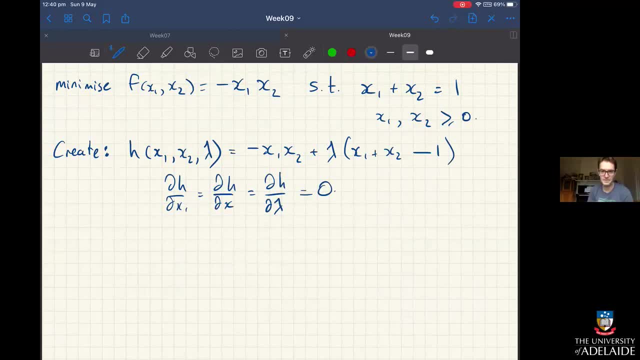 are equal to zero, that will be. that will find me the minimizer subject to this constraint. So always do that. So all we have to do is we have to differentiate this and set everything equal to zero. So dh dx one is going to be negative x two plus lambda. 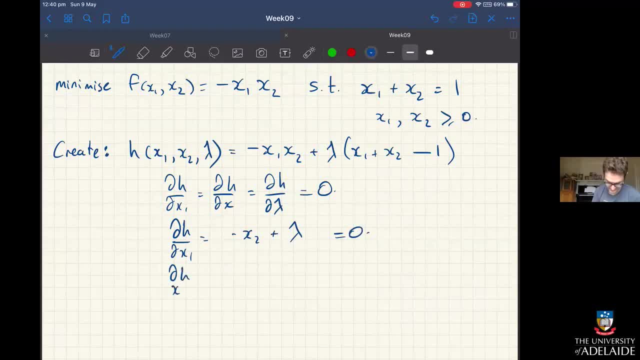 And that's gotta be equal to zero dh dx. two is going to be negative x one plus lambda, And that's gotta be equal to zero dh d lambda. so differentiating with respect to lambda is going to give me back exactly the constraint. 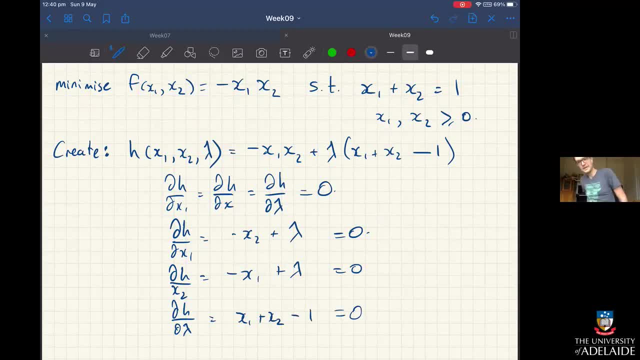 So x one plus x two, take away one has gotta be exactly equal to zero And that's exactly just satisfying that constraint And that should be the case. That's always the case with the Lagrange multiplier problems. and because we have to exactly satisfy that constraint, 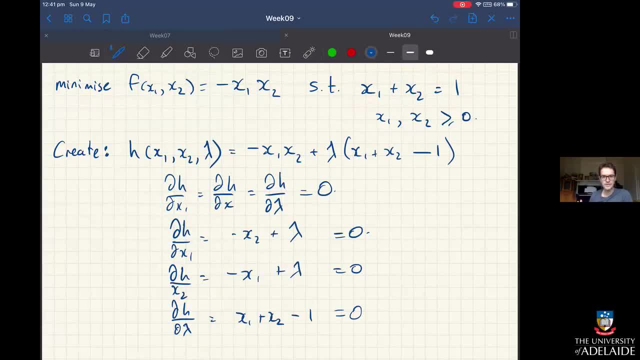 So that's a system of linear equations. So we've got three equations and three variables. I should be able to solve ax equals b. You could do that in MATLAB or you can do that by hand if you want The solution turns out to be. 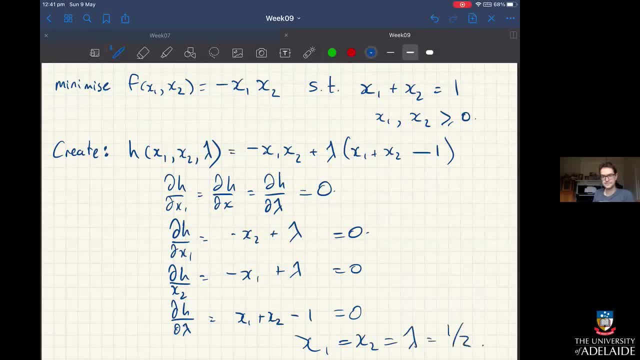 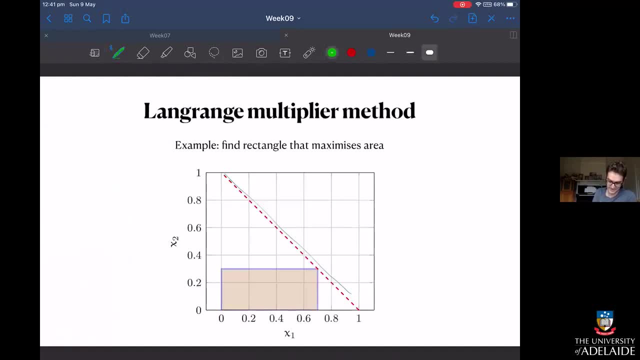 x. one equals x, two equals lambda equals a half, as you might've expected If you just sort of try to guess at the solution here without doing anything. So this: the optimal area rectangle here, is that one Right, that is a square. 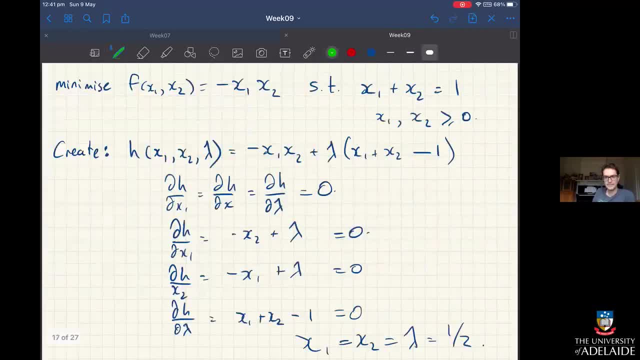 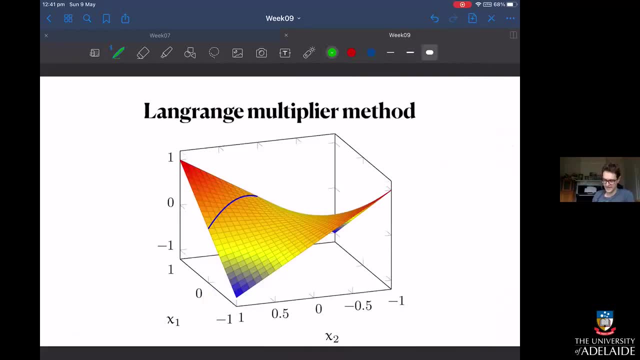 And that's what you sort of expect. So what have we done here? I mean, this is actually the function, This is the cost function f of x one x two that we have been maximizing. So it's not negative, but the function we've been maximizing. 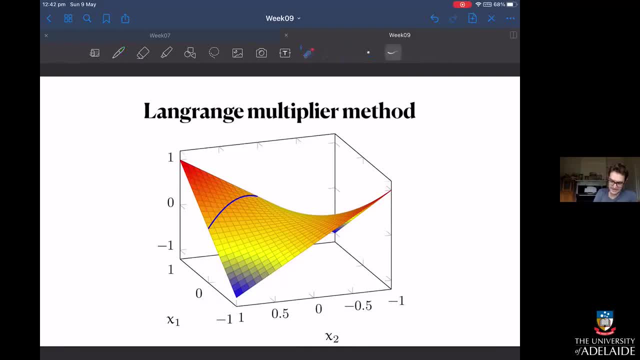 This is the area function in this surface here and this line, and then that's my constraint right. So I was really looking for the maximum of this surface that lies along This blue line that I've just highlighted there. So that's why we find that point that's up there. 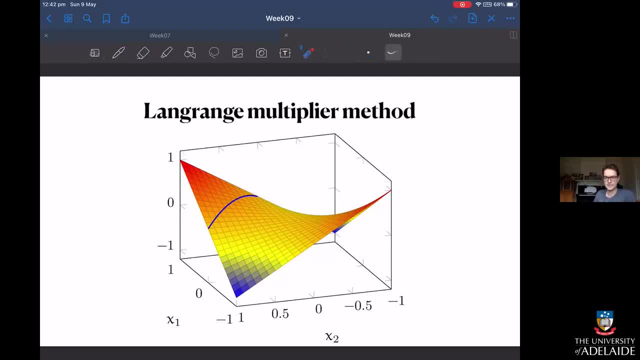 And that's what the Lagrange multiplying method does for us. So that's how it works. So you can do other types of problems here. So you could say: find the area, find the dimensions of the rectangle which maximizes the area inside this circle, right. 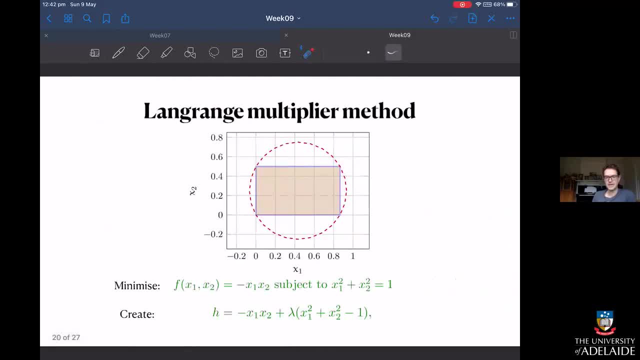 So that's a little bit trickier, But it's the same sort of formalism, right. So we want to minimize in this course, So we'll minimize the negative of the area. So that's still x one, x two, but my constraints now is a little bit more complicated. 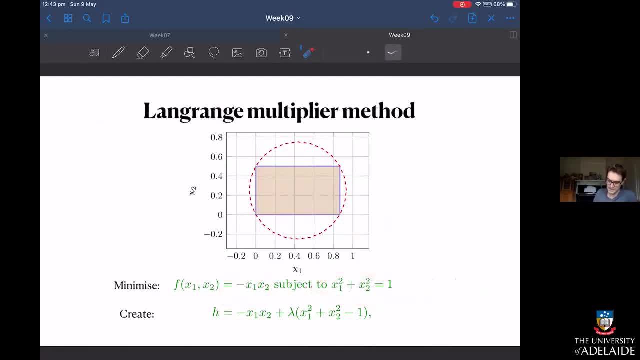 right, It's not a nice linear set of constraints. And now I need that this rectangle. the edges of it lie on this circle, So x one squared plus x two squared has got to be equal to one. So that's a little bit trickier. 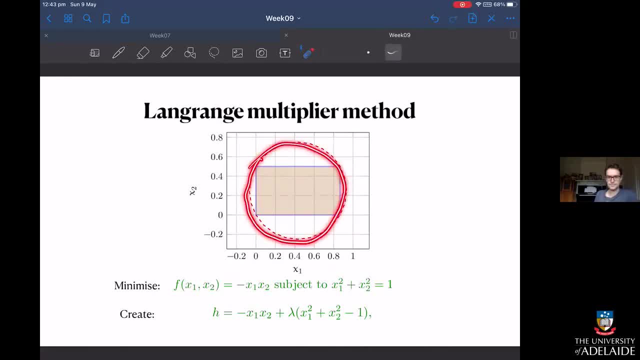 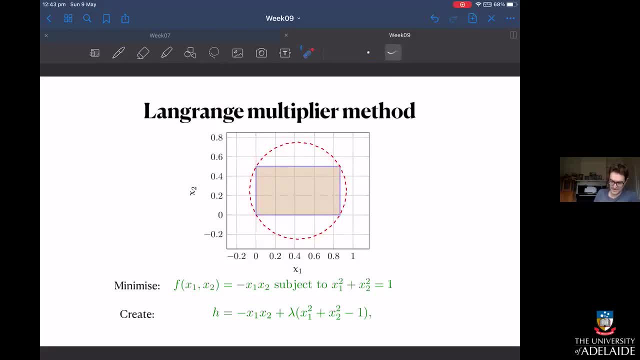 And so that's the problem with its constraint. And so what we do is we write down the same sort of thing. So we create this new function h, which has got my f of x. So that's the same as that plus Lambda times, the constraint. 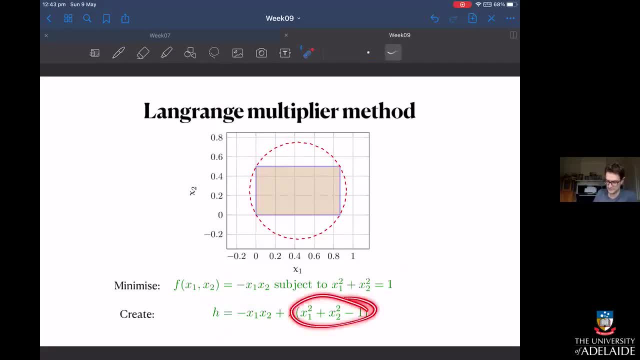 So those two things match up. So when this function is equal to zero, I've satisfied that constraint exactly. So you know that's a little bit more algebraically complicated to do. You're not going to end up with a system of linear equations now. 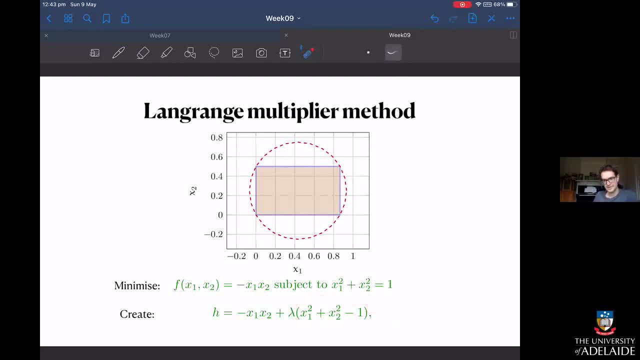 because dh d Lambda is going to have x one and x two squared in it. But the same approach sort of works. You know, you can still work this through and come up with the solution and you get a square again. Becomes a little bit more complicated. 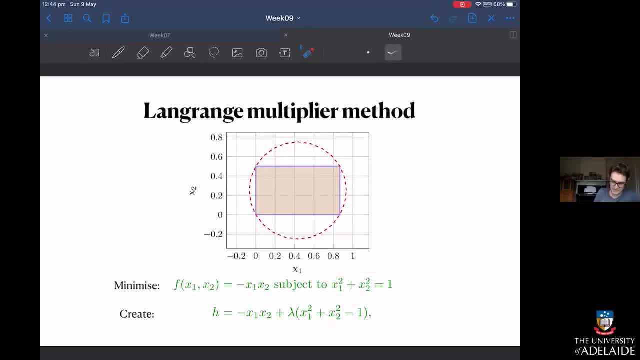 if, instead of a circle here, I make this be an ellipse. So if I divide two by some a squared and some f squared, I'll have b squared here and make this become an ellipse. You can have more fun with that. That's worked out in the notes. 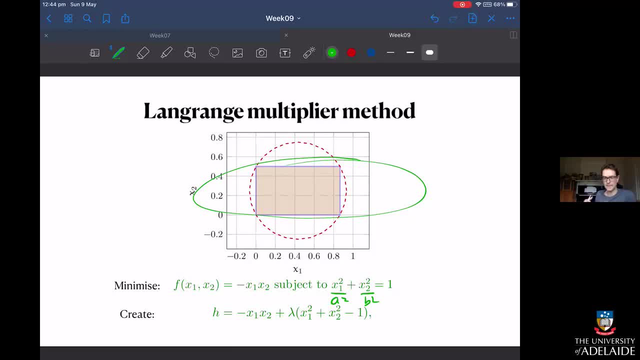 And so you can. you should make sure that you go through the notes and you try these yourself. try to figure them out, check the answers from the notes and go from there, And that's how the method works. So I'll leave you to look through these things yourself. 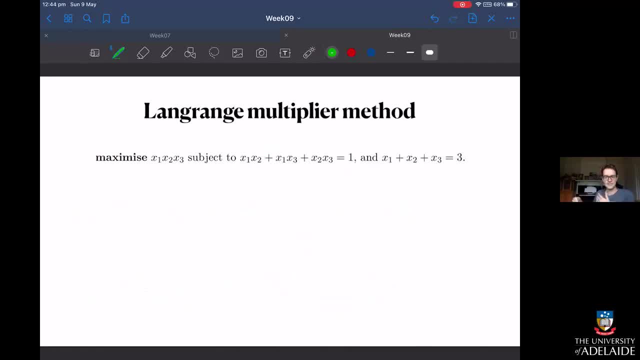 So finally, you know this is a more general method, Right? Like, if you think back to these problems, like you kind of knew how to solve at least problems like this from high school. you didn't need a Lagrange multiplier method to solve this, right? 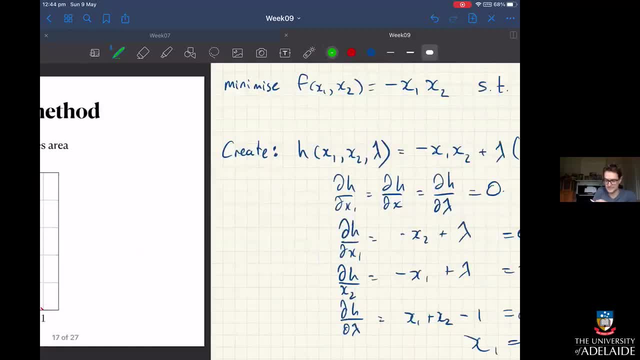 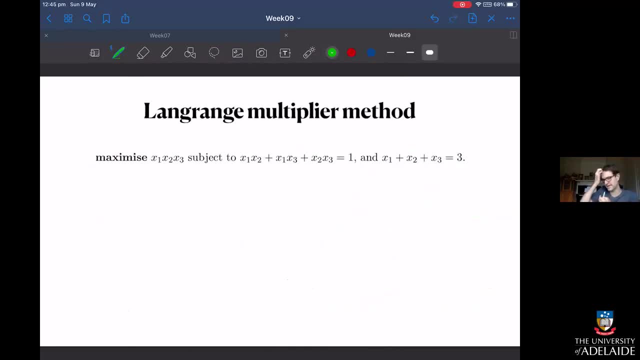 Because you could have figured this out using sort of high school calculus. but you can do much more complicated problems. So here's a pretty relatively complicated optimization problem. So maximize some volume subject to some complex set of constraints. So I've got two constraints here. 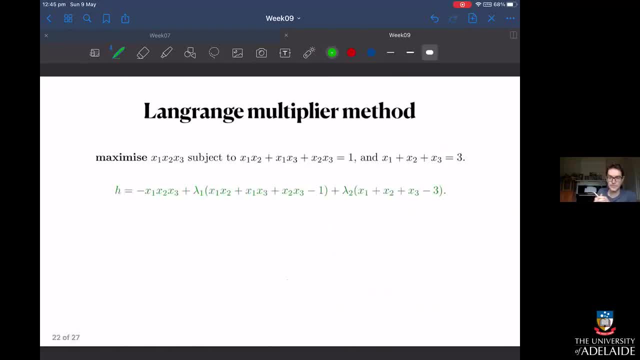 two things that need to be satisfied, And so what we do is exactly the same formalism, right? So we take the thing that I'm trying to maximize, I convert it into something that I can minimize instead, And then each of my constraints go into. 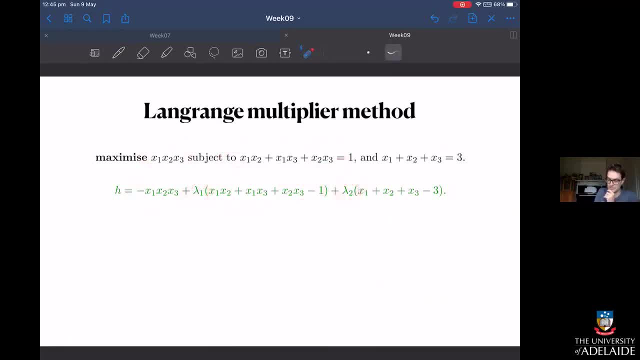 go into that cost function with a Lambda one and a Lambda two, So the second constraint fits in there, and I can put it in as many constraints as I want. And then the problem is: you know, if I want to, you know. 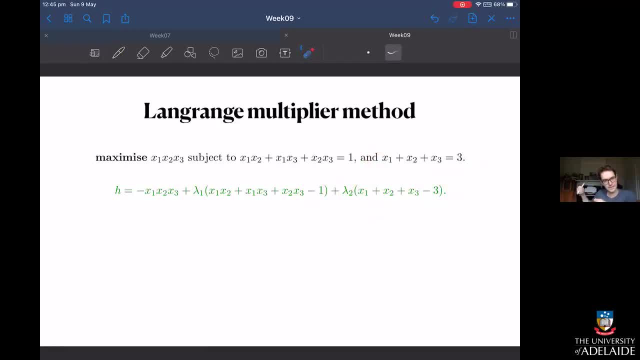 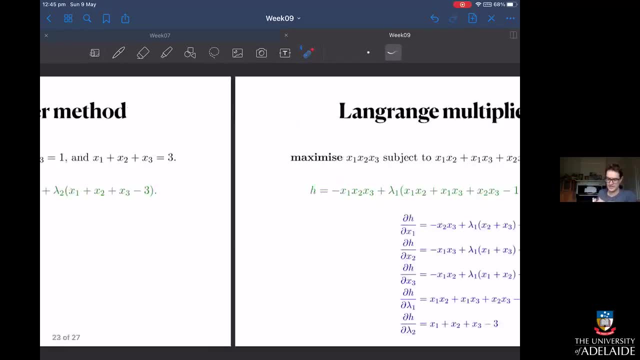 I can put it in as many constraints as I want, And then the process works the same. So I differentiate H with respect to X1,, X2, X3, differentiate with respect to Lambda one and Lambda two. we'll get five equations then. 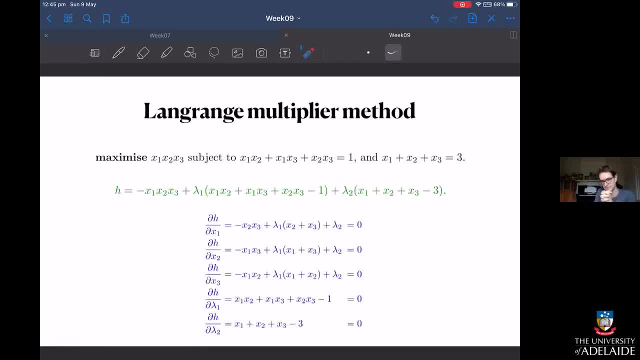 and those are the equations. So the five things I said equal to zero and then you would have to solve those five equations. You know that's really not nice to do now, right Like. so it's not clear how you solve that. 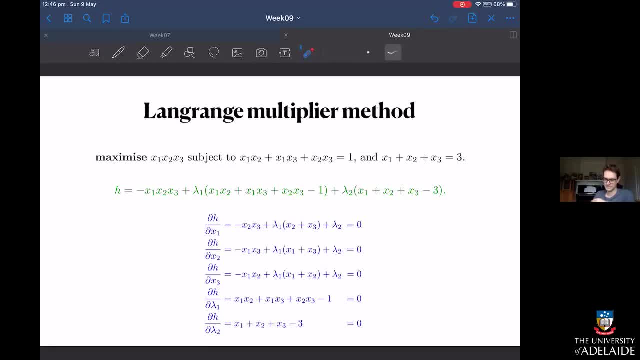 You still need algorithms to now solve that. So you need to have a system of equations, because this is now a really nonlinear set of equations. That's quite ugly. It's got all these nonlinear terms all over the place. But the formalism is there and we can be guaranteed. 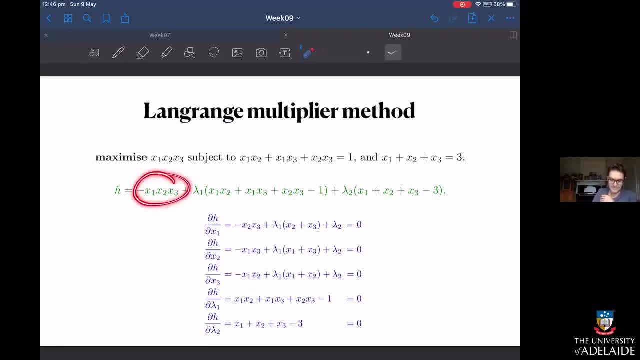 this will find us the minimizer of that function, subject to these constraints. So that's what I want to say about. So you don't necessarily get the solution without you know, using some sort of algorithm words, without needing to do some complex work. 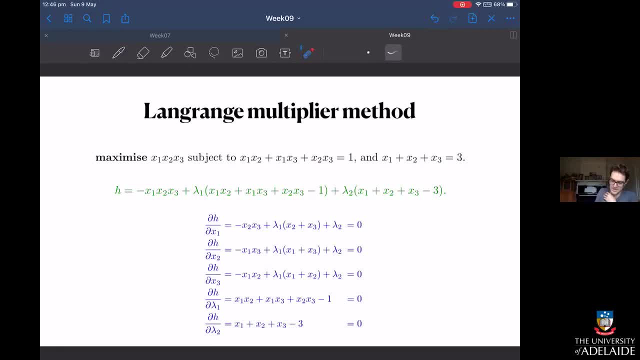 but it gives you a formalism for solving any of these problems that have equality constraints. Okay, so that's a little grunge multiplier method. Just a couple of comments about this. So you know, demanding that all of these partial derivatives of my new cost function H, 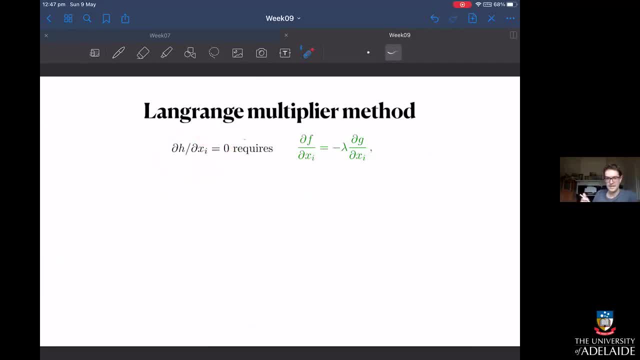 demanding that they're equal to zero. if you chase it through, that means that I'm demanding that the derivative of F with respect to XI are equal to negative Lambda of the derivatives of the constraint functions, And that's because of the way I set up this cost function. 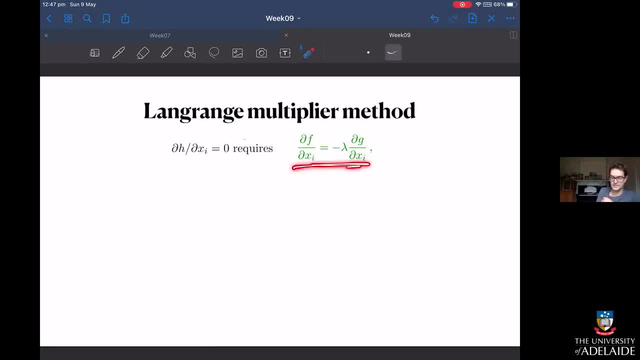 So you know, solving the problem requires this result here and actually a more concise way of putting that. I've written that with index notations. but I'm really saying that the gradient of F is equal to negative Lambda times the gradient of G. 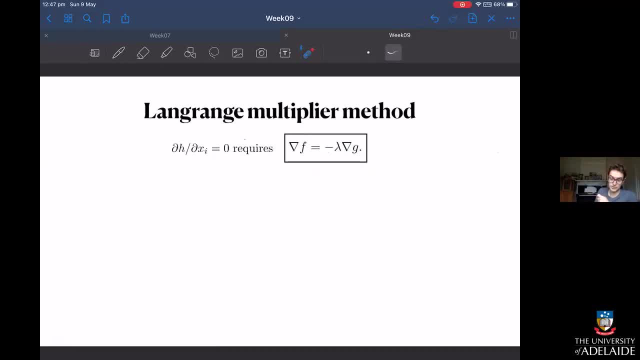 where G is my constraints, my vector of constraints here, And so that's actually a really important point about these things. So yeah, so you can see that you know. here's an example where the brown lines represent level curves of my cost function. 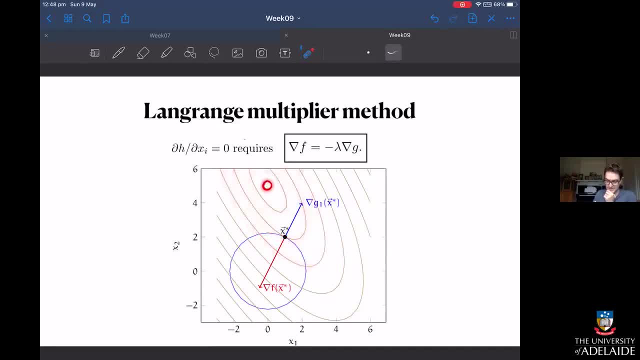 So you can see that I'm trying to minimize the function F, right? So the overall minimizer of that is somewhere in the middle here And my constraint G is the circle here. So I'm trying to minimize over this region, minimize the brown function over this region. 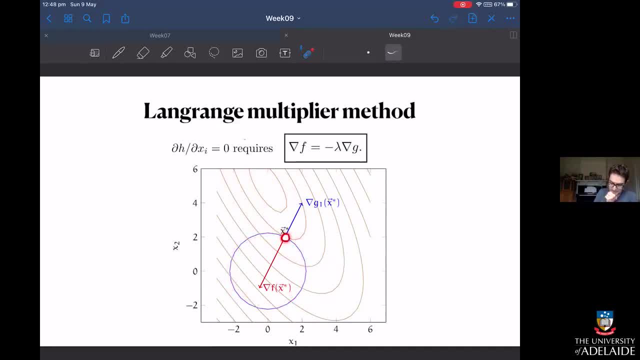 but subject to being on this blue line here, right, And so the minimizer of that is going to occur here, And so the gradient of F- right, So that's the direction of steepest ascent at this point away from the minimizer- has got to be equal to the negative. 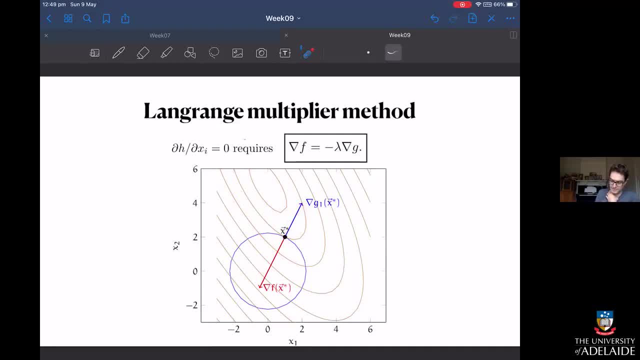 over scaled version of the gradient of the cost function. sorry of the constraint here. So you know, this is the fact that this, this new watching, a type of, and this vector point in opposite directions. there's not an accident, right. 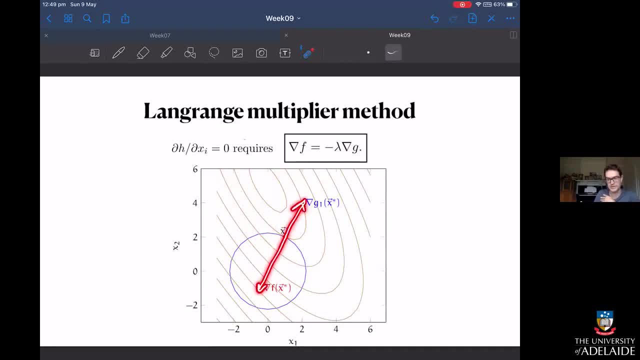 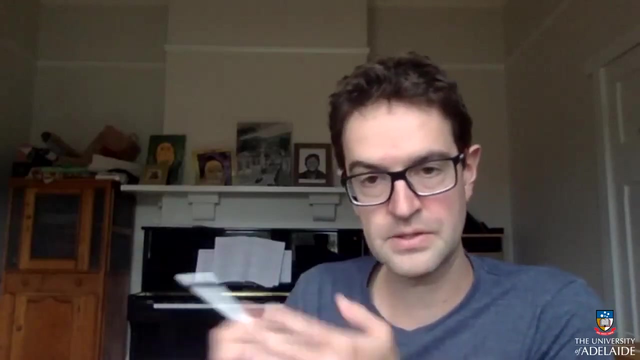 minimizer. you know, the that direction points in the opposite direction to that and that's an important result. and actually this little, this little result here, when we take the next step and start to talk about constrained optimization and with inequality constraints, and that point becomes, becomes really important. so, and that's all I'll say about Lagrange multipliers, what I 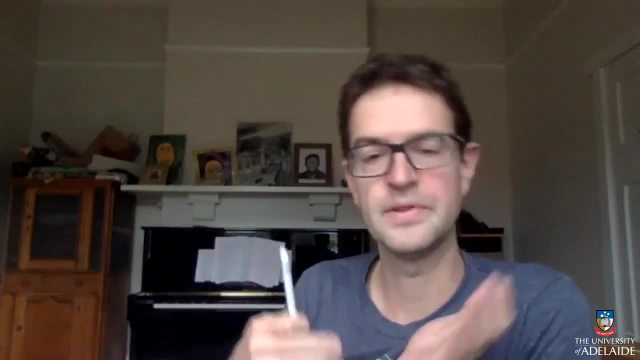 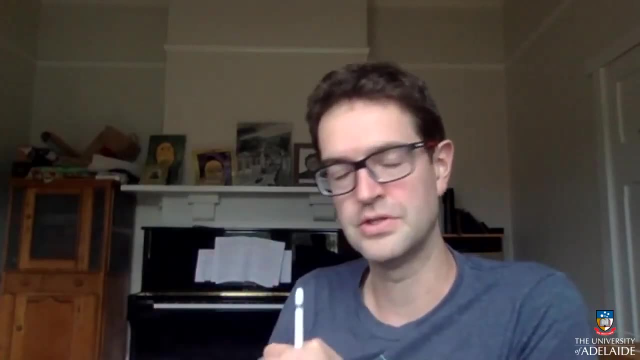 want you to do is I want you to go and check out the examples that I've just shown you in the notes and work through them yourself and and check the work solutions that are in there. so make sure that you can do all of those processes and yeah, and then we'll move on to talking about inequality. 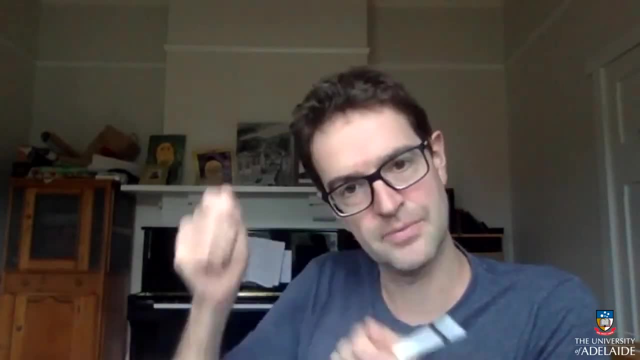 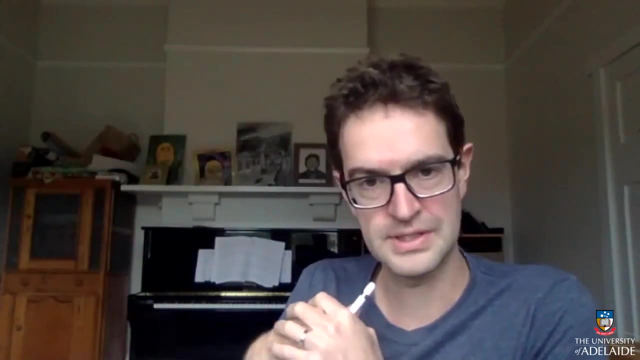 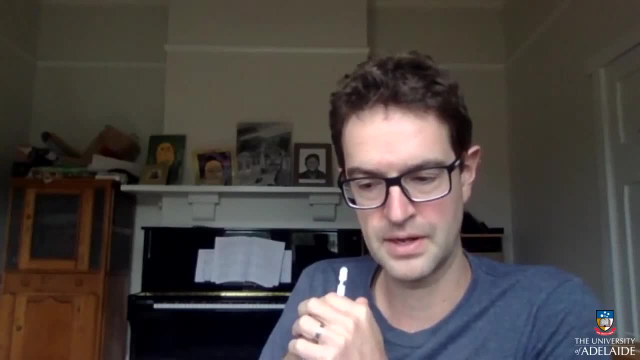 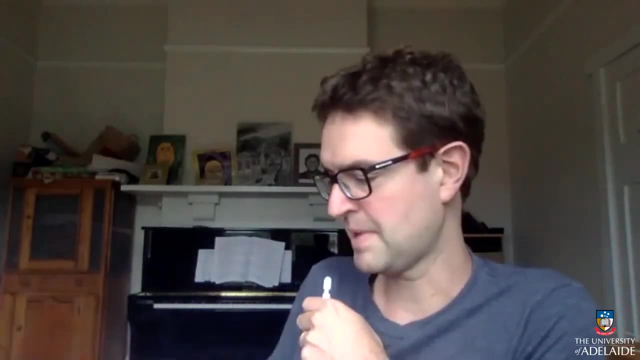 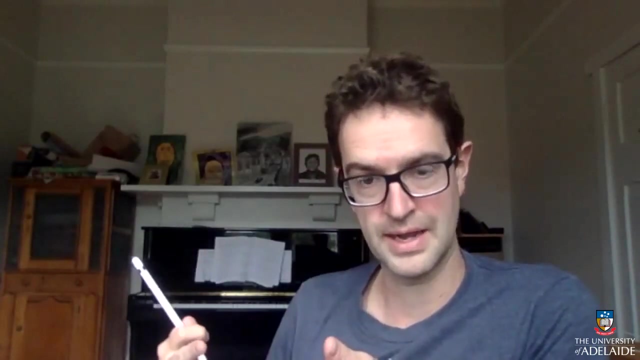 you know Lagrange multipliers for for us, as a method for solving constrained optimization problems. I should mention that they're really important in other parts of, in other parts of science, so in physics, so in mechanics, the whole field of Lagrangian dynamics, so you can solve.